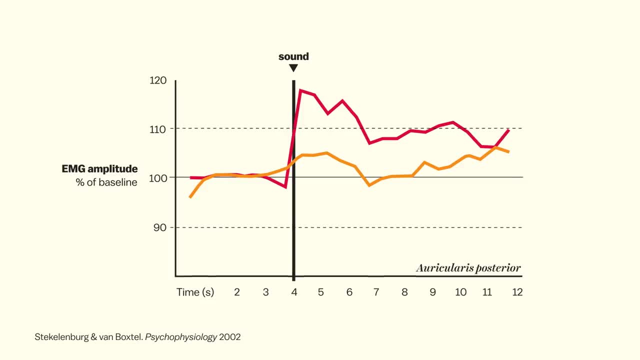 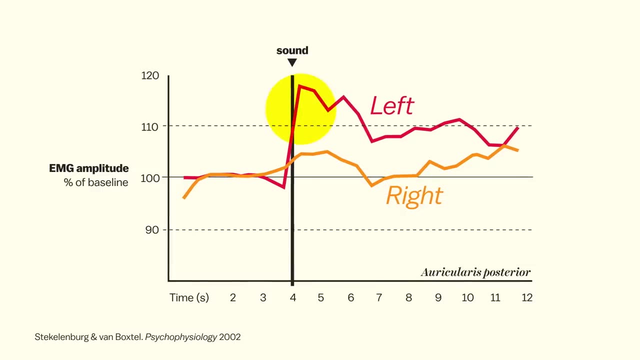 Not enough to move the ear, but detectable, And you can probably guess the location of the sound based on these results. It came from a speaker placed to the left of the study subjects, So this is their left ear, subconsciously trying and failing to pivot toward the sound. 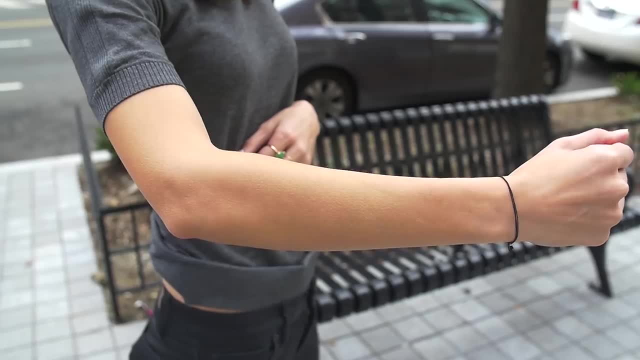 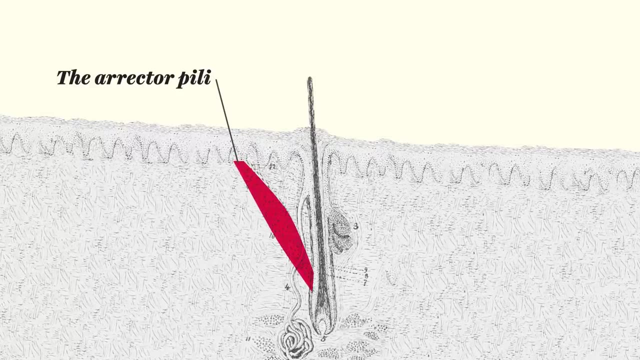 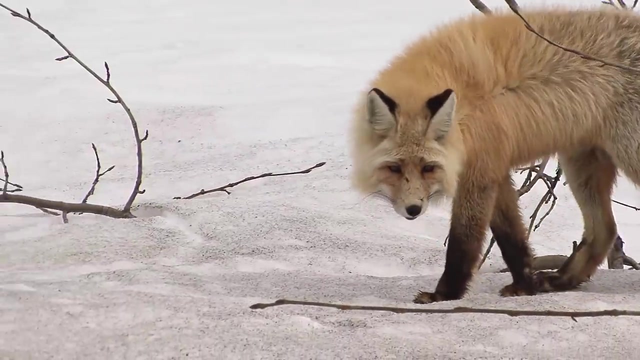 You can see another futile effort by our vestigial body parts when you get goose bumps. When we're cold, tiny muscles attached to our body, hairs contract, pulling the hair upright which causes the surrounding skin to form a bump For our furry mammal relatives. the raised hair increases the amount of space for insulation. 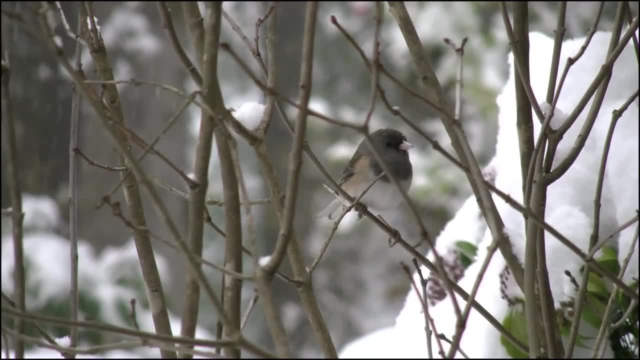 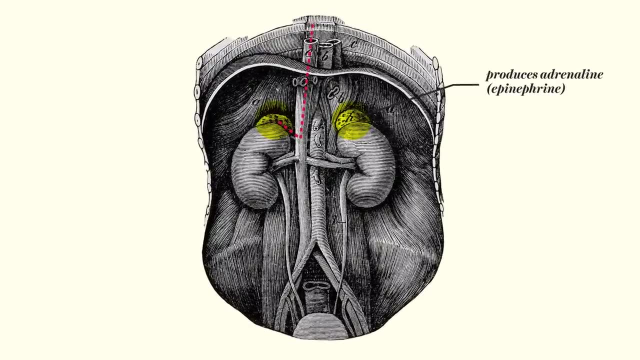 helping them stay warm. Birds can do this too. You've probably seen a puffy pigeon on a cold day. Adrenaline is one of the hormones involved in the body's response to cold temperatures, and it's also part of the fight or flight response. 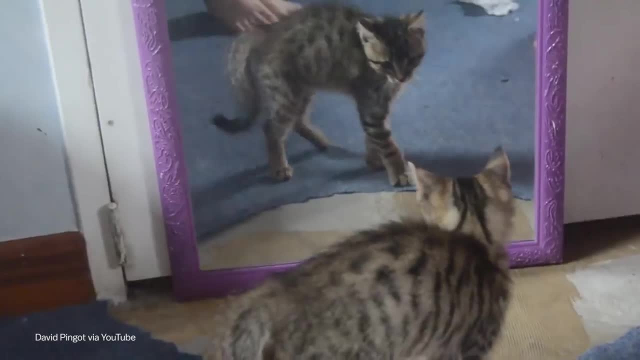 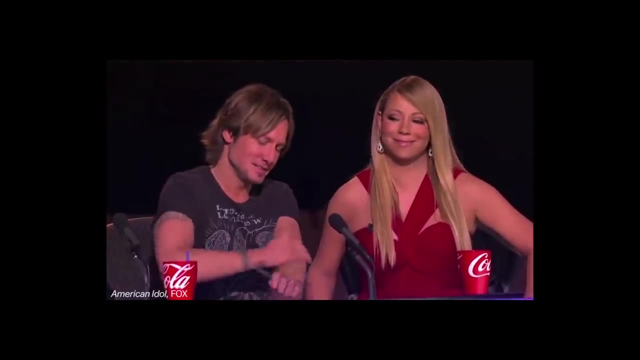 So it helps. some animals appear larger when they're threatened, And it may be why surprising and emotional turns in music can give some people goose bumps. And then there's our tail: At the end of our spine are a set of fused vertebrae. 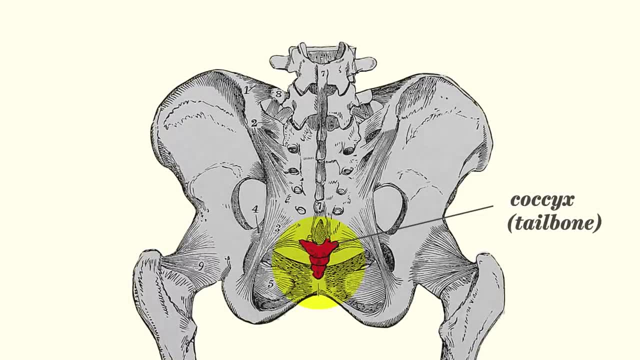 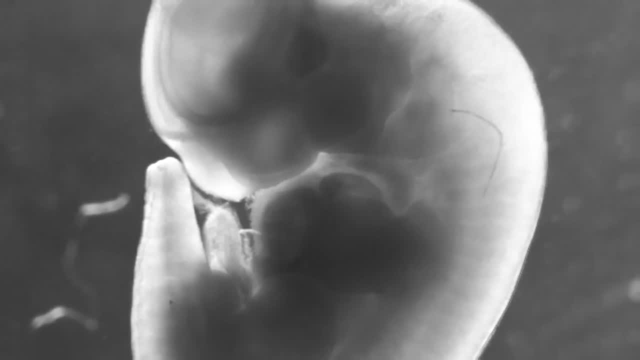 Some people have three, some people have five. We call it the tailbone. It now serves as an anchor for some pelvic muscles, but it's also what's left of our ancestors' tails. Every one of us actually had a tail at one point. 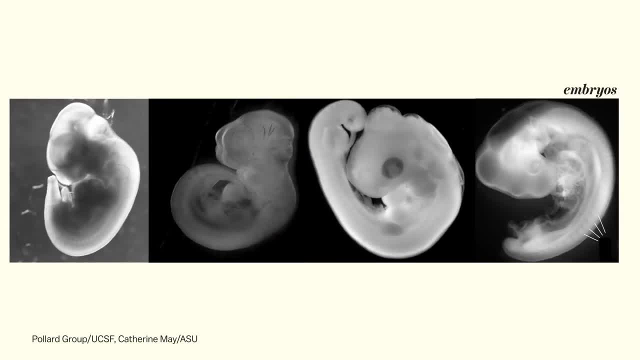 When the basic body plan is being laid out at around four weeks of gestation. human embryos closely resemble embryos of other vertebrates, And that includes a tail with 10 to 12 developing vertebrae. In many other animals it continues to develop into a proper tail. But in humans and other apes the cells in the tail are programmed to die a few weeks after they appear. Very rarely, though, a mutation allows the ancestral blueprint to prevail and a human baby will be born, A baby will be born with a true vestigial tail. 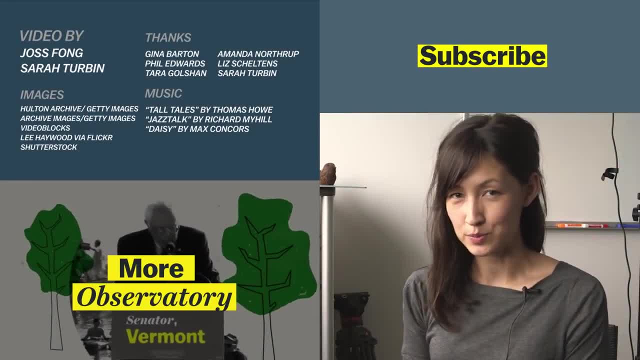 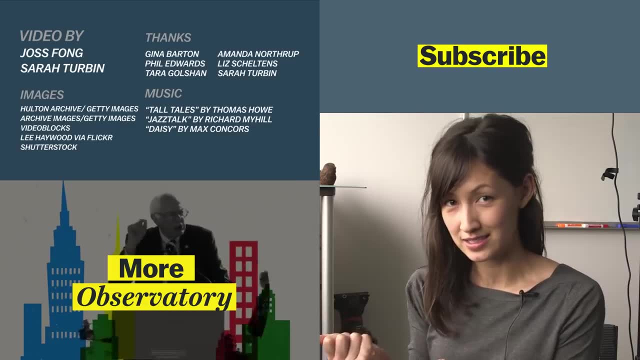 The most adorable vestigial behavior is the palmar grasp reflex, where infants up until they're about six months old have this incredible grasp on whatever you put in their hand. There's a similar reflex for their feet. I wanted to show you this great piece of footage from the 1930s. 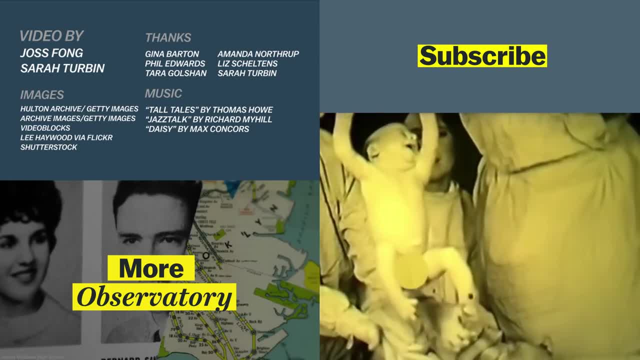 where they demonstrated this behavior. These babies are only one month old and you can see that their inner monkey is able to support their entire weight.